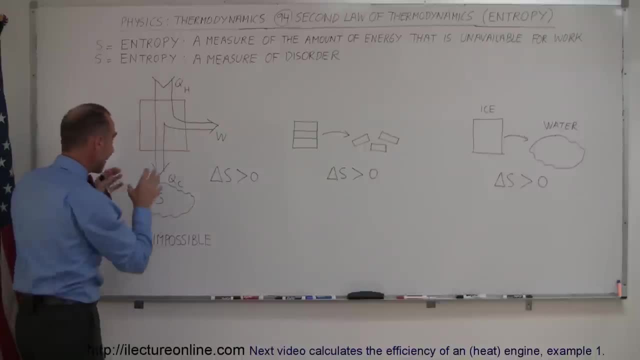 heat flow from a hot reservoir to a cold reservoir. Once heat ends up in the cold reservoir, you can do work with it. relative to the hot reservoir, You'd have to take that heat and bring it back up here, And that of course requires work and input of work to get that done, So on its own that will never. 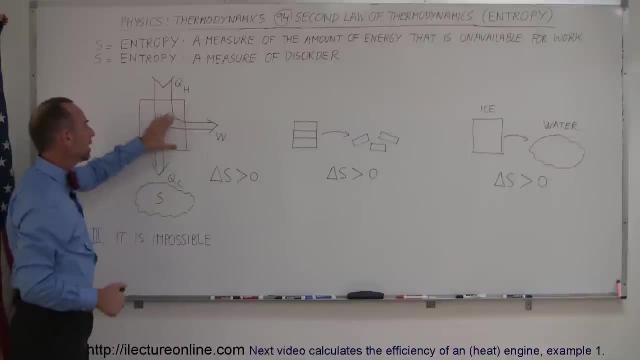 happen. So, because doing work with a heat engine requires heat to flow from a hot to cold reservoir, more and more heat enters the heat engine, And that's what we're going to talk about today, And that's what we're going to talk about today. Therefore, more and more, 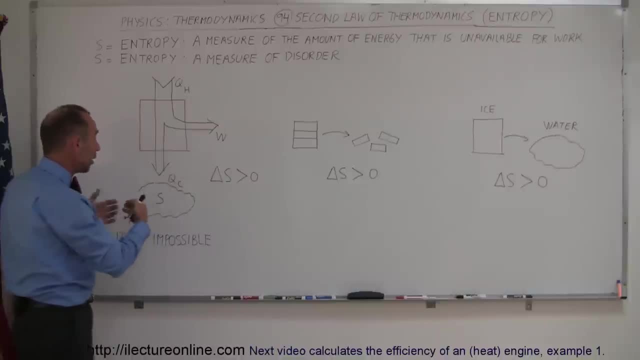 unavailable energy, or I should say more and more energy unavailable to do work with. So, therefore, the entropy S- We use the letter S for entropy, I don't know why, but there it is, And so the change in entropy is always going to be positive. Again, that's the amount of energy unavailable for work. 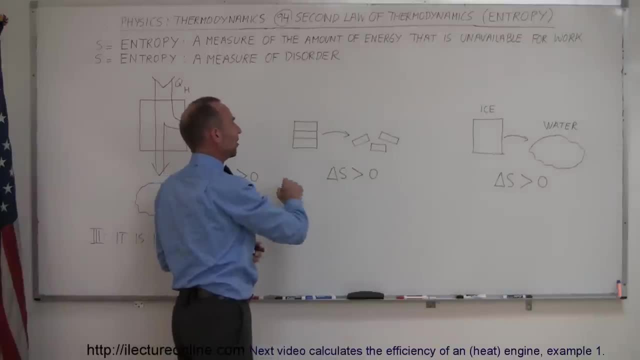 Another way of looking at it is: we have these bricks nicely stacked up. Someone comes along, kicks them over, or the wind comes along, Kicks them over and they all fall down. Now we're in a less ordered state and therefore this has lower entropy and this has higher entropy. So the changes from low to high, therefore, the change is: 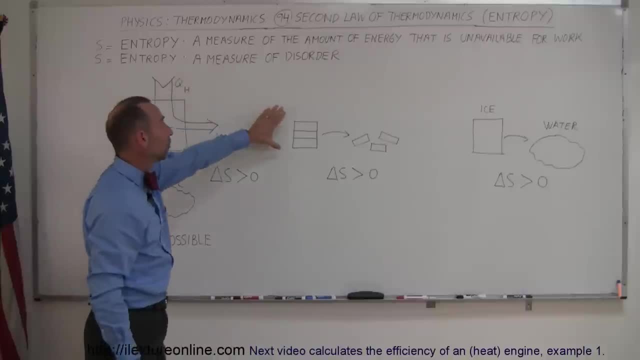 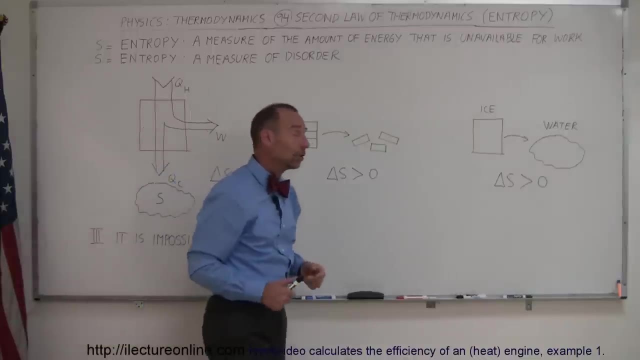 positive. That refers to this run right here. We call this a more ordered state and we call this a less ordered state. Less order means higher entropy. And here another example. let's say we have a block of ice. Heat comes along, starts heating up the ice, The ice begins to melt, turns. 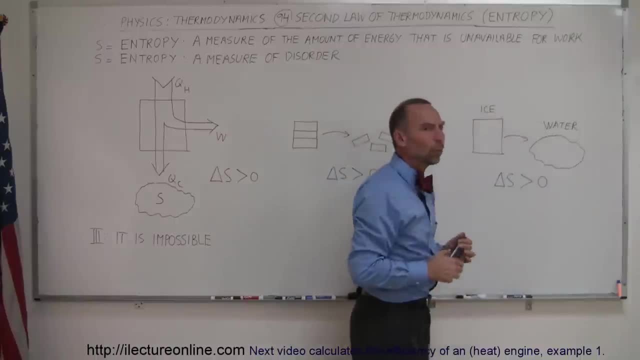 into water. This is a more ordered state. This is a less ordered state, And one way to look at it is: here: all the water molecules are locked into a crystalline lattice, So they're very well ordered in a cube, And once it becomes water, they just go everywhere. They roll over each other. So this is. 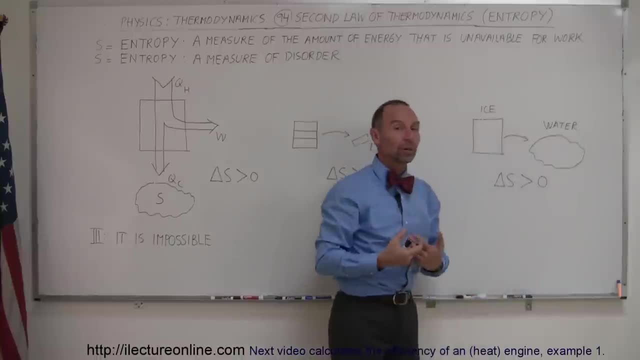 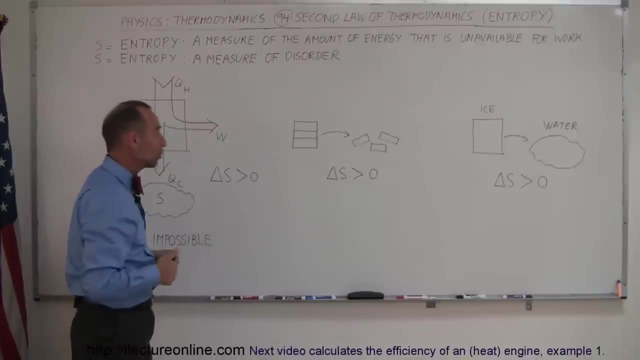 higher order, lower order, Entropy goes up because we're in a less ordered state. So you can see that in any process that happens on its own, entropy tends to increase. So how do we express the second term of thermodynamics in terms of entropy? It is impossible in a thermodynamic process for